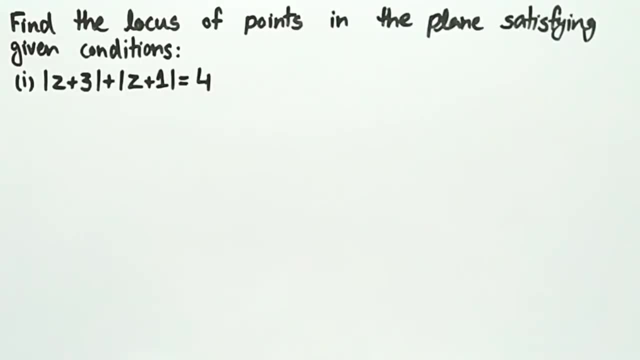 In this video we will discuss two examples in which we will find the locus of points in the plane satisfying given conditions. First one is mod of z plus 3 plus mod of z plus 1 equal to 4.. Firstly, we will put z equal to x plus iota y and we get mod of x plus iota. 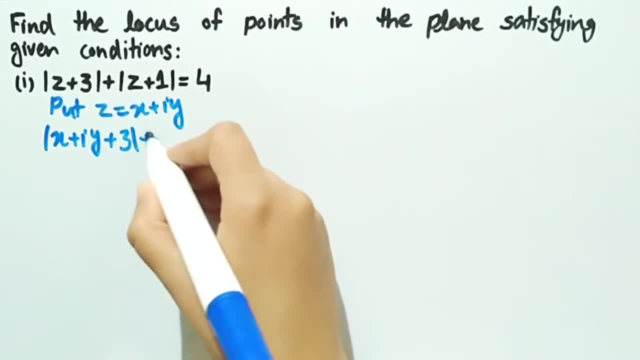 y plus 3 plus mod of x plus iota y plus 1, equal to 4.. Now we will rearrange it and write it as mod of x plus 3 plus iota y plus mod of x plus 1 plus iota y, equal to 4.. Now 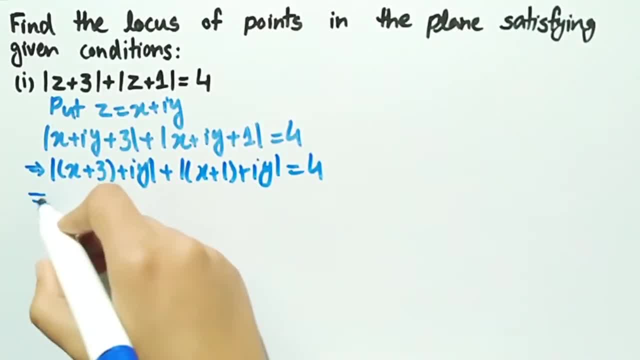 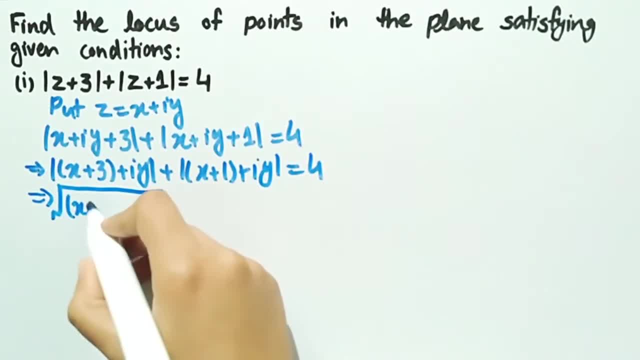 root square of real part, that is x plus 3. square plus square of imaginary part, that is y square plus mod of x plus 1 plus iota, y will be equal to square root of real part, that is x plus 1. square plus square of imaginary part, that is y square equal to 4.. 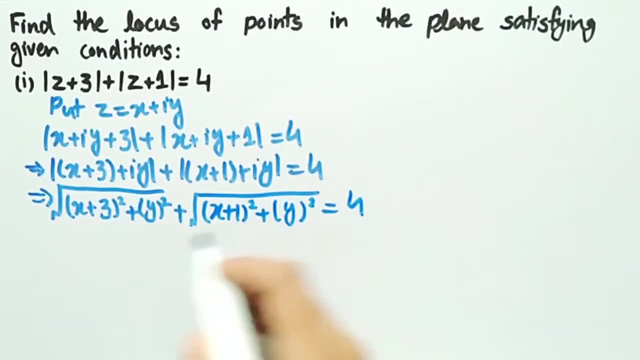 Now transferring this term on the other side of equality, we get square root x plus 3 whole square plus y square, equal to 4 minus square root x plus 3 whole square plus y square, equal to 4 minus square root x plus 3 whole square. 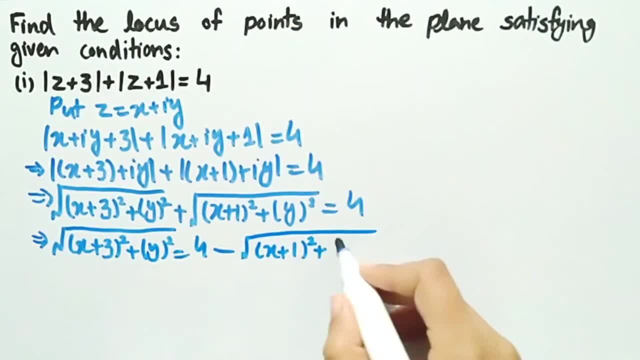 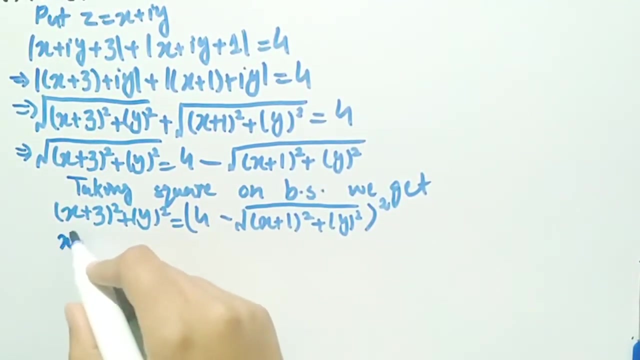 plus 1 square plus y square. now, taking square on both sides, we get x plus 3 whole square plus y square, equal to 4 minus square root. x plus 1 square plus y square, whole square. x plus 3 whole square is equal to x square plus 9 plus 6 x. 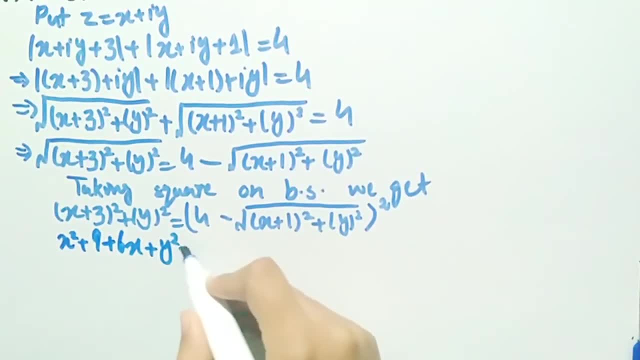 and y square square is equal to y square, equal to now. we will take the square of this term and it will be equal to 16 plus x plus 1 whole square plus y square minus 8 square root x plus 1 whole square plus y square. now we can also write it as x. 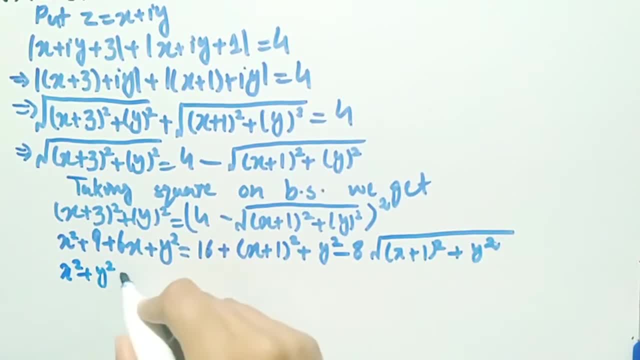 square plus y square plus 6x plus 9, equal to 16 plus x square plus 1 whole plus 2x. this is the square of x plus 1 whole square plus y square minus 8. square root: x plus 1 square plus y square. we can rewrite it as x square plus. 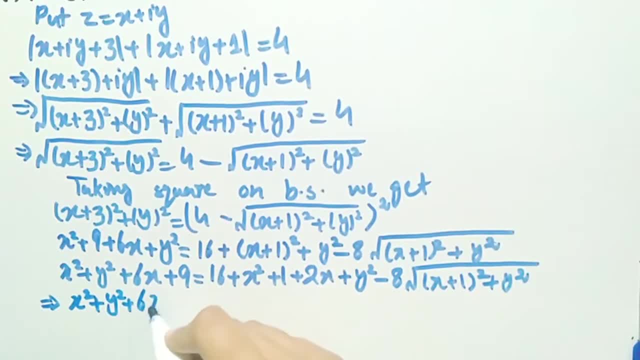 y square plus 6x plus 9. now transferring these terms on the side of equation, we get minus 16 minus x square, minus 1, minus 2x minus y square, equal to minus 8 square root, x plus 1 whole square plus y square. 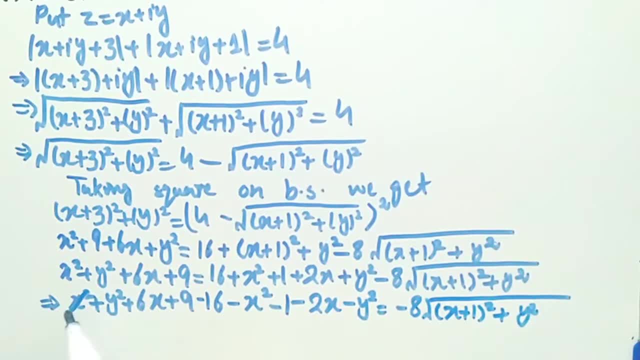 this x square will be considered to be x plus 1 whole square plus y square. understood x square will be considered to be now for the next step星野만 will be out by minus x square plus y square will be cancelled out by minus y square, 6x minus 2x. 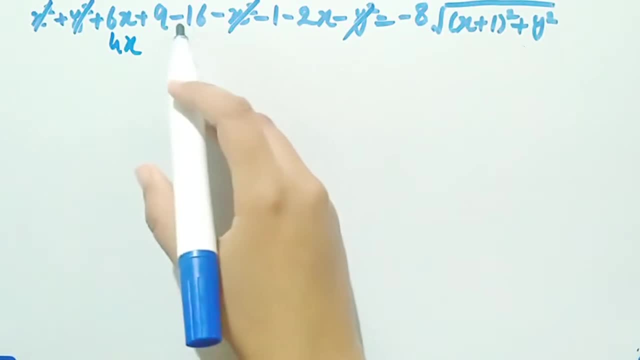 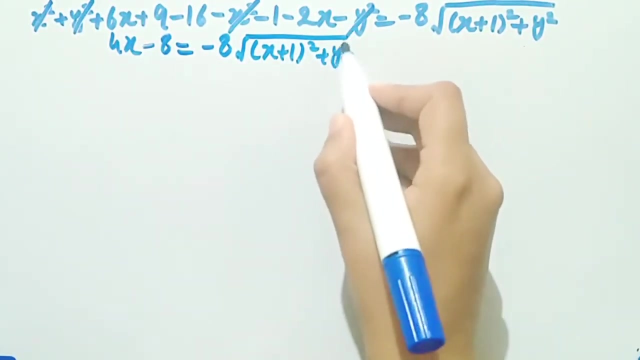 is equal to 4x, and 9 minus 16 minus 1 is equal to minus 8, which is equal to minus 8 times square root, x plus 1 square plus y square. Now, dividing this equation with 4, we get dividing both sides. 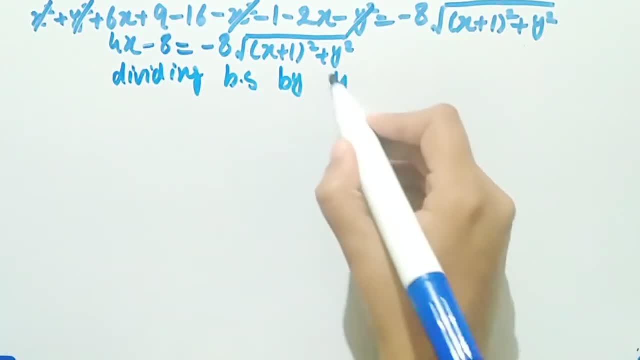 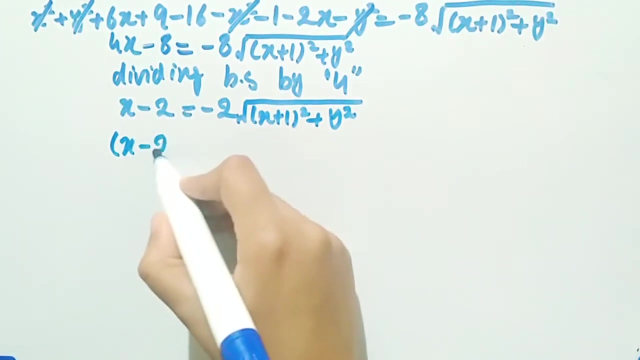 by 4, we get x minus 2 equal to minus 2. square root x plus 1 minus 2. square root x plus 1 square plus y square. Now, dividing this equation with 4, we get square plus y square. now, taking square on both sides, we get x minus 2 whole. 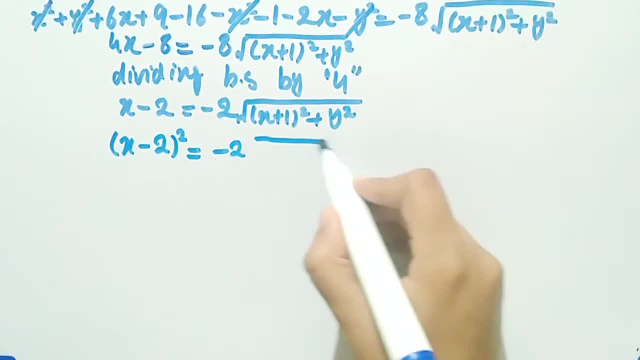 square equal to minus 2 square root x plus 1 square plus y square whole square, and it will be equal to x minus 2 whole square is equal to x square minus 4x plus 4 and it is equal to 4x plus 1 square plus y square. we can rewrite it as x square minus 4x plus 4. 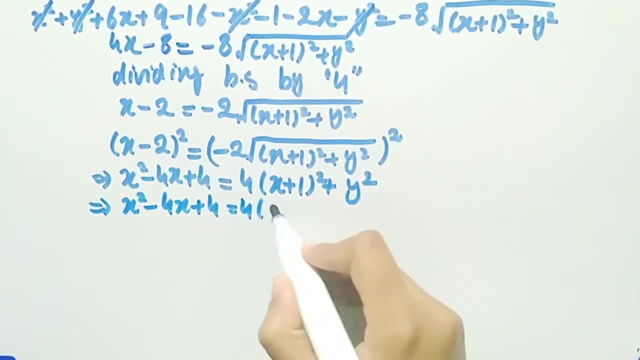 equal to x minus 2 whole square and it will be equal to x minus 2 whole square is equal to to 4 times x square plus 2x plus 1 plus y square, which can be written as x square minus 4x plus 4, equal to 4x square plus 8x plus 8 plus 4 plus 4y square. Now transferring all of these, 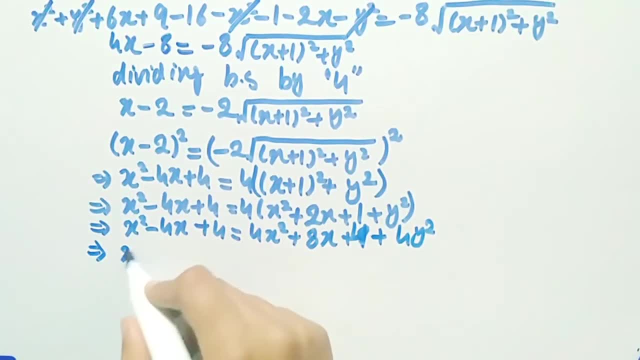 terms to the left hand side of this equation, we get x square minus 4x plus 4 minus 4x square minus 8x plus 4y square. 8x minus 4 minus 4y, square equal to 0.. This 4 will be cancelled out by minus 4 and we are: 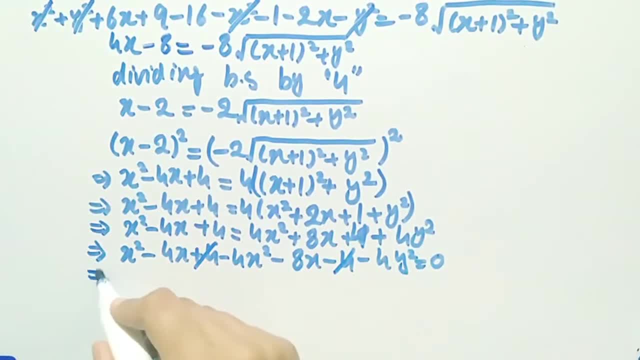 left with x square minus 4x square is equal to minus 3x square, and minus 4x minus 8x is equal to minus 12x. 8x minus 4 minus 4y square equal to 0.. Now, multiplying this equation by minus 1, we get: 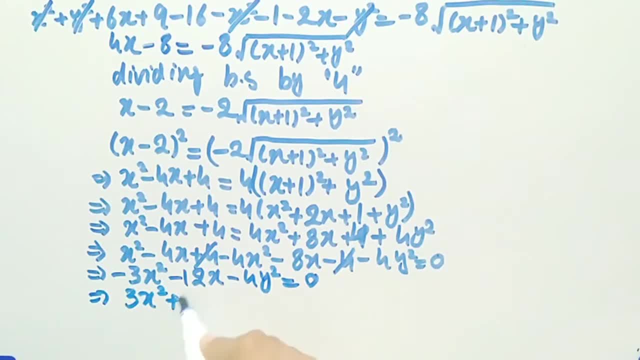 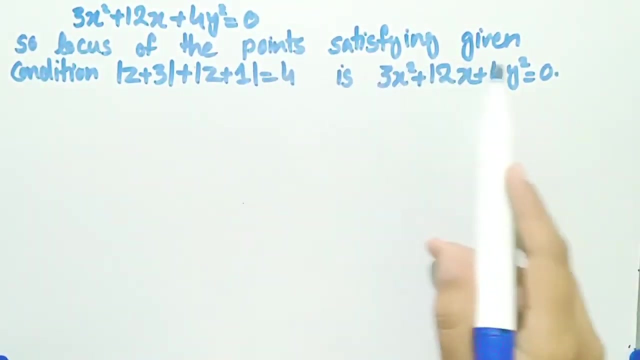 3x square plus 12x plus 4y square, equal to 0.. Now we have to write the equation of the points satisfying given condition: mod of z plus 3 plus mod of z plus 1, equal to 4, is 3x square plus 12x plus 4y square, equal to. 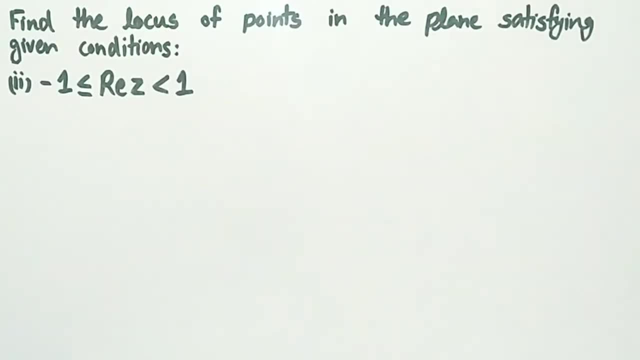 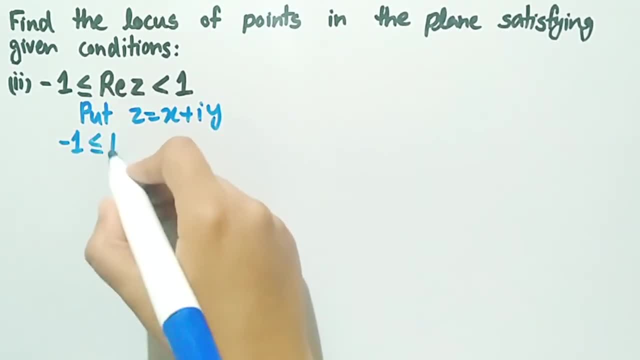 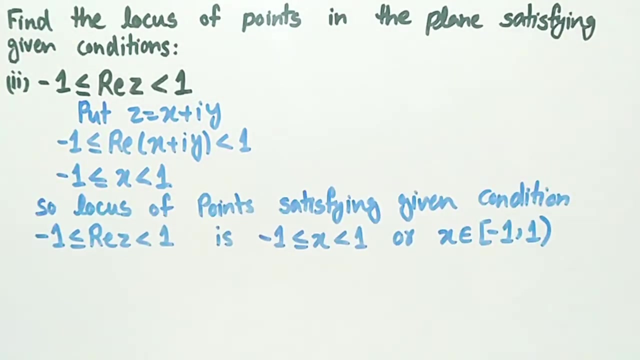 minus 1 is less than equal to real part of x plus iota y less than 1.. We know that real part of x plus iota y is x, so we can write it as: minus 1 is less than equal to x is less than 1.. So, locus of points satisfying given condition, minus 1 less than equal to x is: 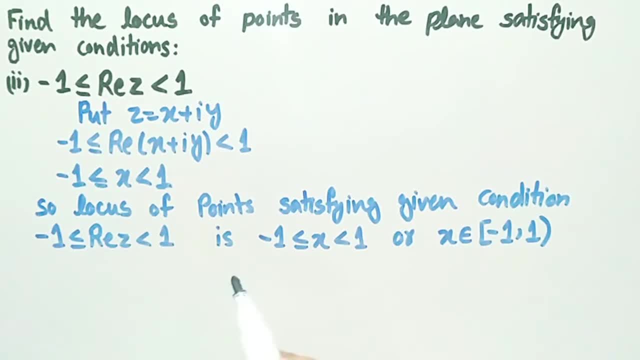 less than equal to real part of z. less than 1 is minus 1. less than equal to x, less than 1 or half open, half closed interval minus 1: 1, such that x belong to this interval.